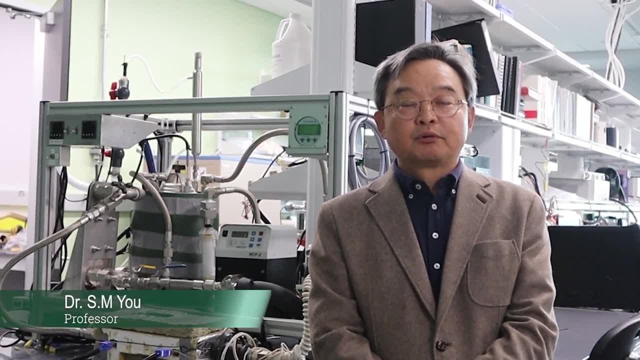 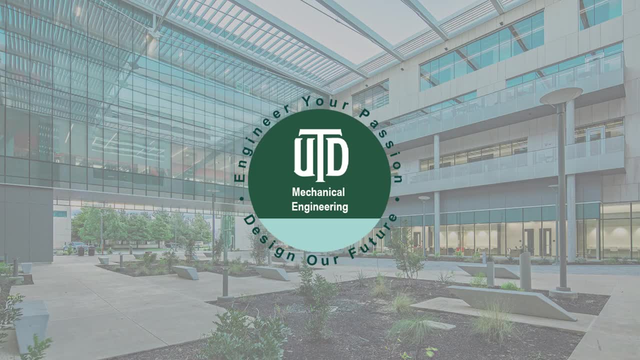 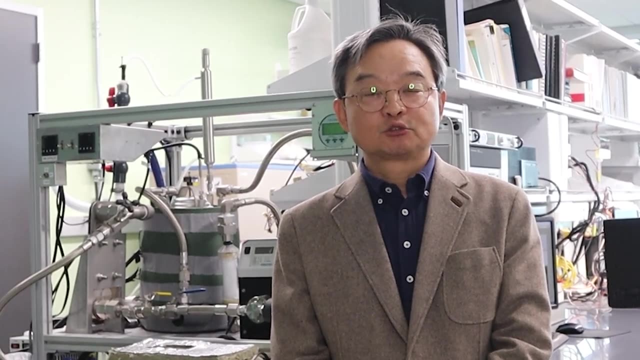 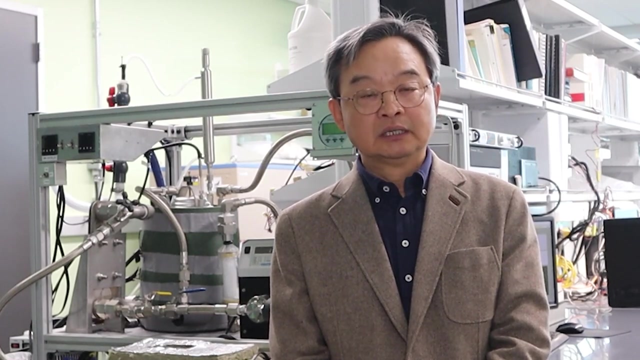 Hello, I am Dr SM Yoo, professor of mechanical engineering at the University of Texas at Dallas. My lab is focused on doing a research to enhance multi-phase heat transfer problem and we utilize these different scales, including micron scale and nano scale, and the application is also broadly. 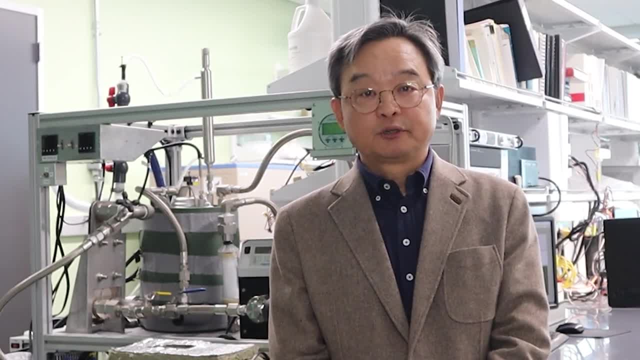 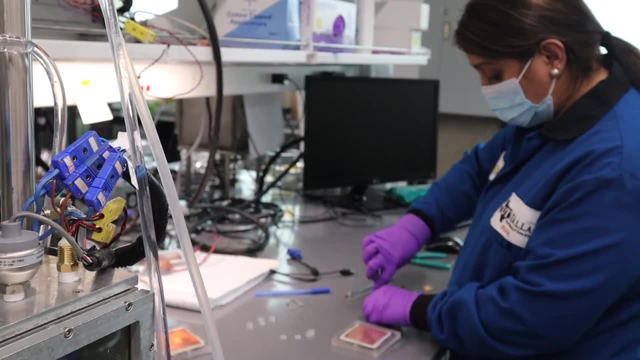 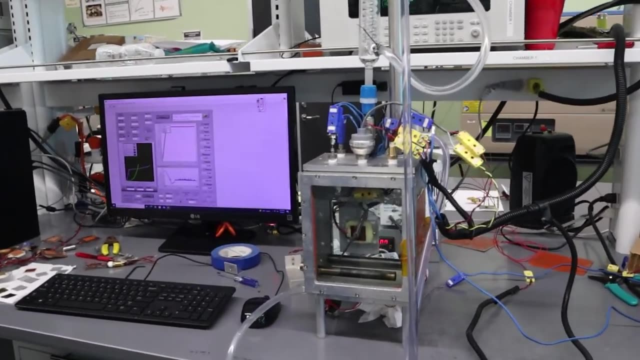 ranged, and the first one could be such as very small ones like a smartphone, up to the nuclear accident cooling situations. In those applications we use two key technologies we invented in the lab. The first one is called micropolar surface coating. What it does is providing micropolar structures. 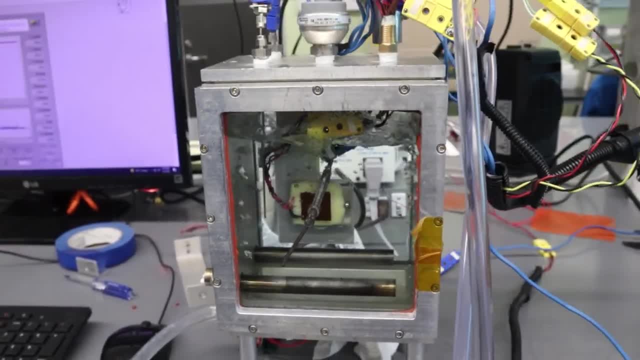 of about 100 micron thickness, so that, if you don't have the coating, we only see the one bubble compared to the other one. If you don't have the coating, we only see the one bubble compared to the other one. If you don't have the coating, we only see the one bubble compared to the other one. 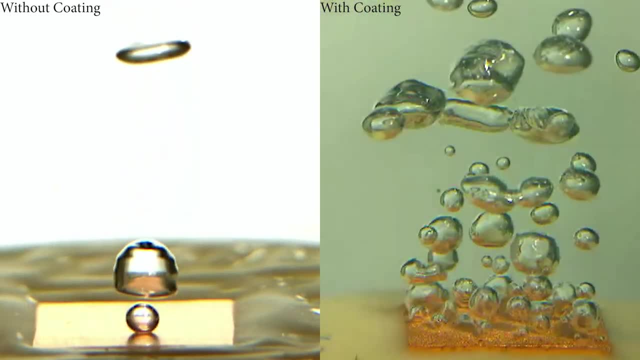 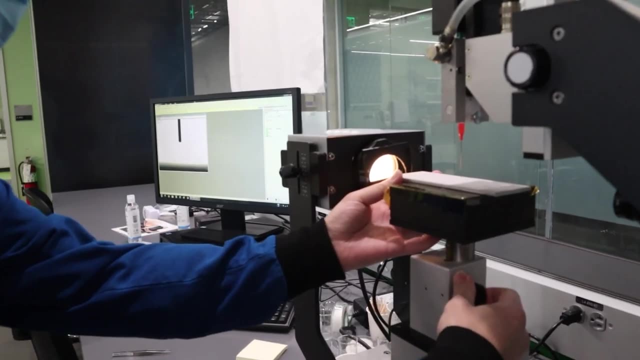 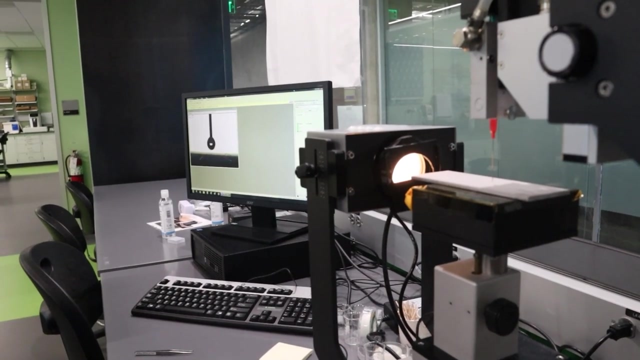 Micropore coated surface provides hundreds of bubbles on the surface and which causes very efficient cooling on the surface. The other coating is called nano scale surface coating, which could provide broad ranges of wettability: extremely wetting versus extremely non-wetting. Therefore, when you have an extremely 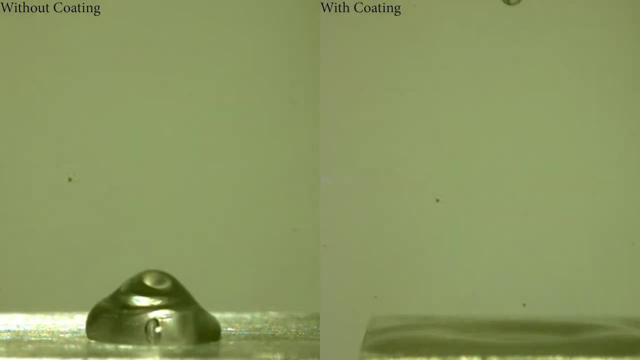 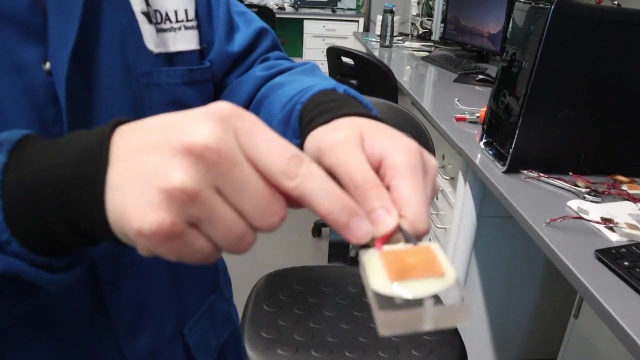 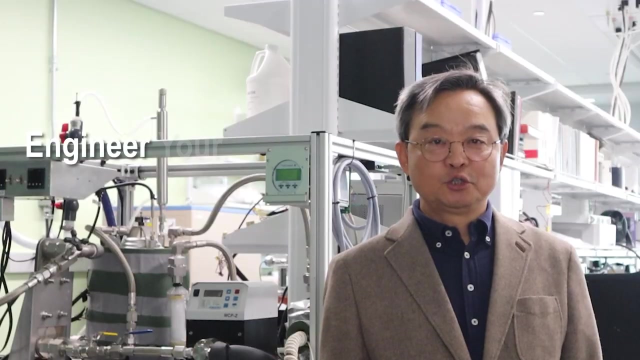 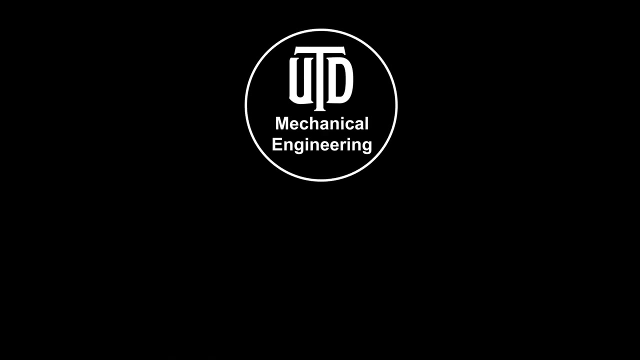 wetting condition, it spreads the liquid into a wider area, such that the evaporative heat transfer is more resilient. When it's non-wetting, then we can effectively collect condensation drops. Engineer your passion, Design our future.